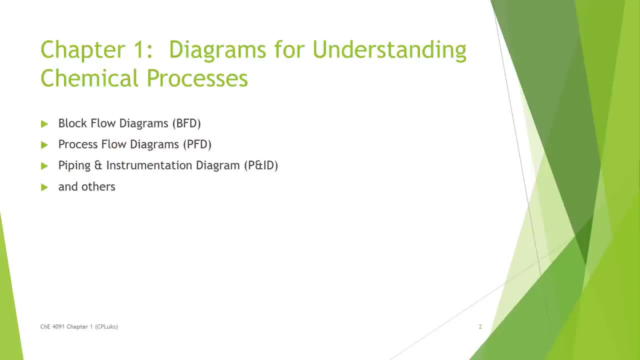 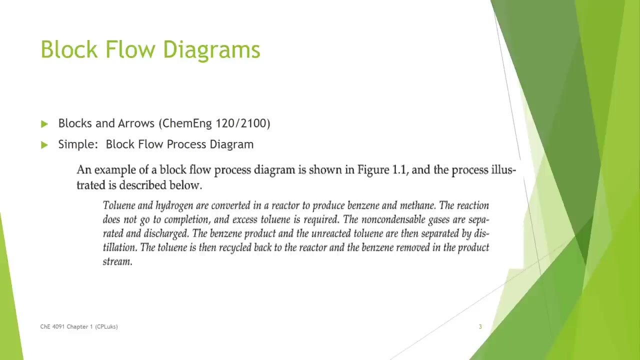 So a block flow diagram is a BFD, A process flow diagram is a PFD And a piping and instrumentation diagram is a PNID. Block flow diagrams are the typical blocks and arrows that you learned back in chemical engineering 2100 when you did your mass and energy balances. 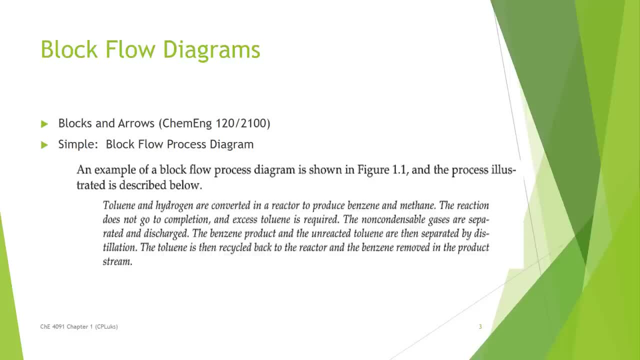 And they can be really, really simple. We have material coming in, something happens to it, that's the block, and then material comes out, And so here, toluene and hydrogen are converted in a reactor to produce benzene and methane. 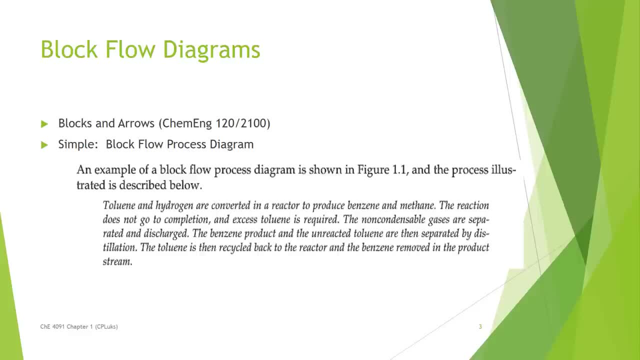 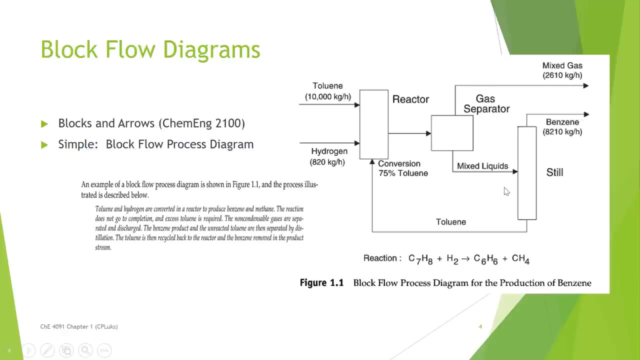 And they give us more information about that. But if you do this, what you see is that toluene and hydrogen come in, benzene and methane are being produced and the leftover toluene and hydrogen come out. This then could be separated and we end up with a diagram for this scenario. 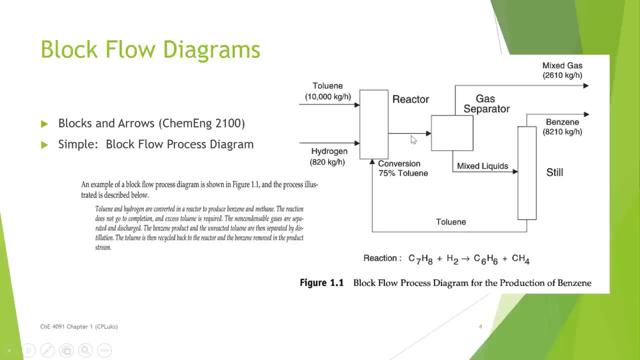 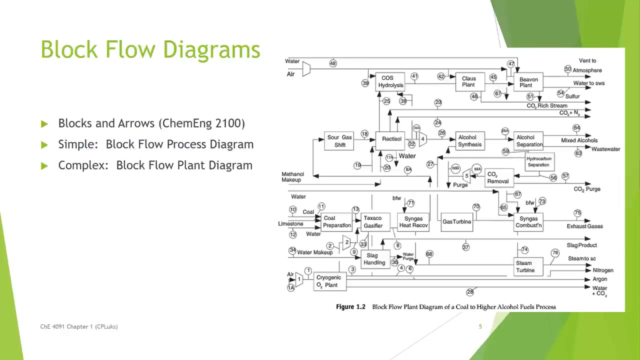 that looks something like this: Two streams in, one out, but it needs to be separated. Some of that material is product benzene, and some of it is going to be sent back into the reactor. So there we have the sort of diagram that we've been looking at since you first became a chemical engineer. 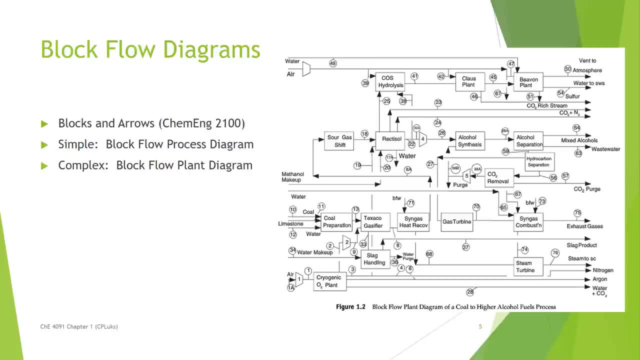 They don't have to be that simple, though. We can have much more complex systems. So this is for producing higher alcohol fuels from coal, And you see that this is much more complicated, but we're still doing the blocks and arrows technique. 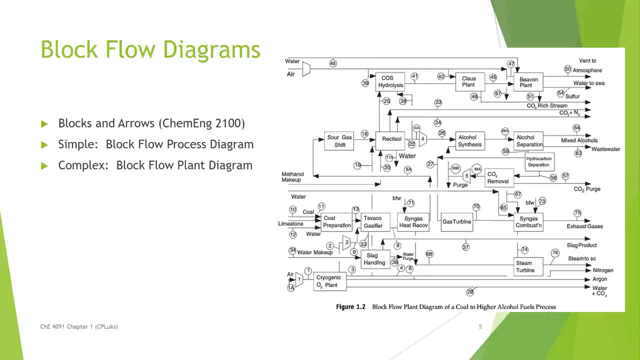 And it's all flowing left to right and it's fairly easy to read. We're told that, like we have a Klaus plant, but it doesn't tell you what the equipment is. It tells you nothing about sizes, It just simply allows you to identify what is happening. 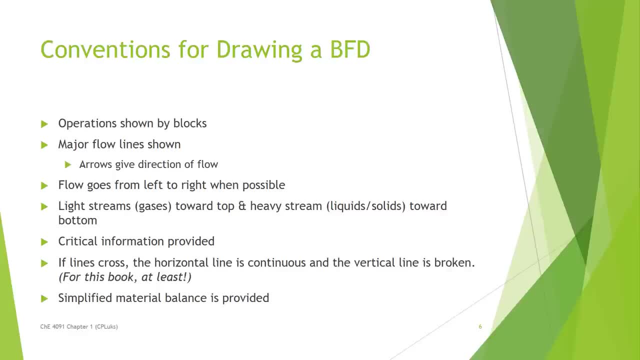 So we show the various operations in blocks. The major flow lines are shown and the arrows are drawn in there to tell you which direction the material is flowing. And the flow is going to always go from left to right if possible, except for, obviously, on recycle streams and so forth. 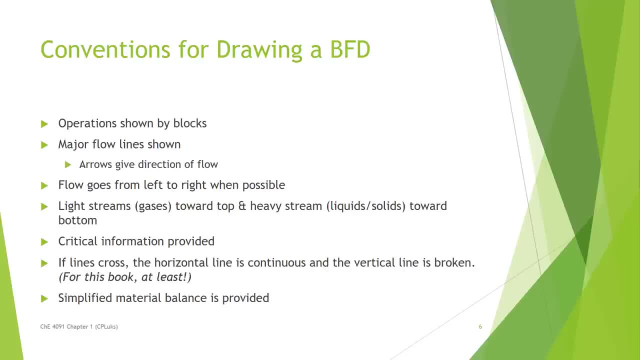 When I have multiple streams going in or out of a block, I typically do the lighter streams at the top and the heavier streams at the bottom, So gases would be at the top, liquids solids down towards the bottom, based on really volatility. 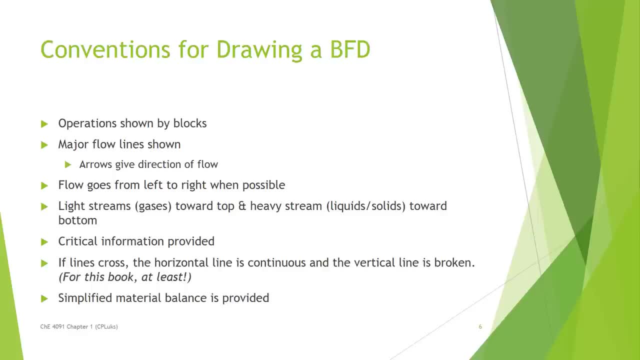 I'm going to put the most critical information on there, Probably going to provide a simplified material balance. Sometimes the streamlines have to cross, and so the way you can do this is you can either do it so that you do a little bump in the line. 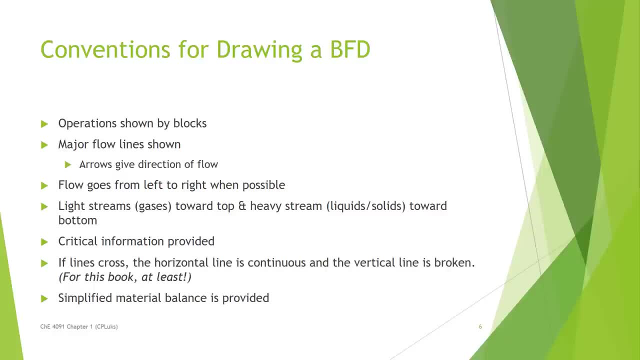 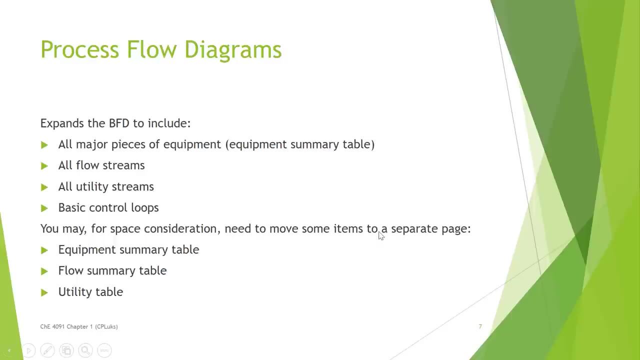 to indicate it's jumping over like a bridge, or they will do the horizontal line continuous and then this textbook. they do the vertical line as broken to indicate that it's going through Now if you want to expand BFD to another line. 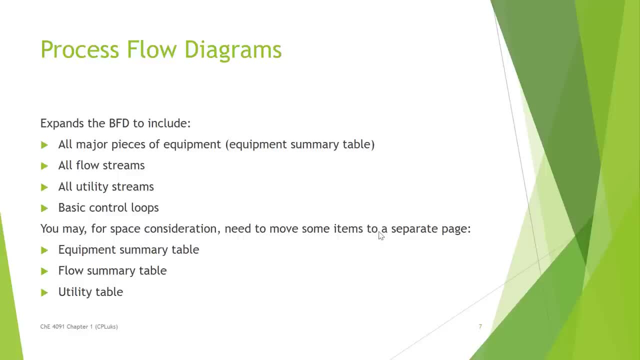 BFD to a process flow diagram. we're going to now include all of the major pieces of equipment. We're also going to be sure that we include all of the flow streams and all of the utility streams. So if I'm using steam to heat something or as a driver for some piece of equipment, 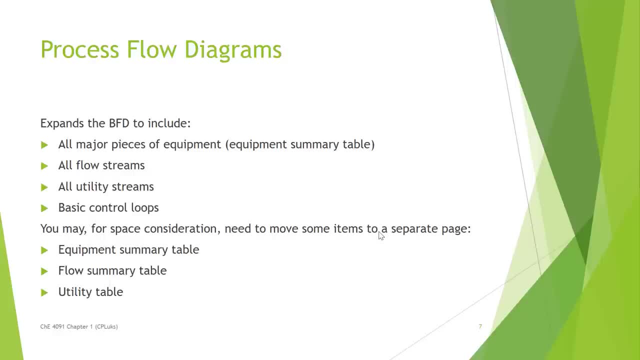 I need to include those, And you also can include the most basic of control loops, but certainly not all of those not exhaustive. Now, sometimes we have to move items to separate pages that would normally go on there, because these things tend to be very, very detailed. 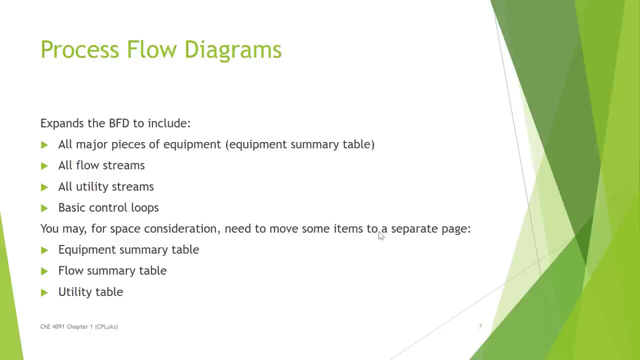 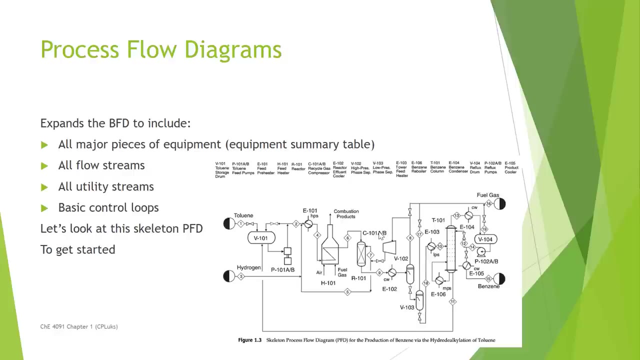 Lots of information on there, And so we will move these things to separate pages, And so you want to always give indicators of what's being moved there, But a lot of the tables that are part of the process flow diagram frequently end up being moved, just for clarity. 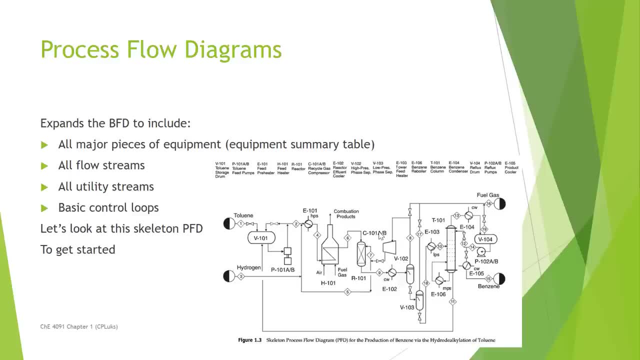 So this is an example that's in your textbook. This is the hydrodealkylation of toluene, and that's an example that they frequently use in the book, And so you'll see here that now then, they're bringing in material and they're showing that it's going into this vessel. 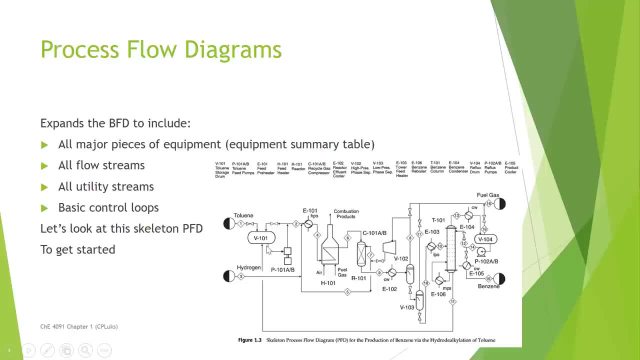 which is the toluene storage drum. So they've identified it up here And then it goes into a pump, And then it goes into an exchanger, And so every piece of equipment is identified in all of the flow streams. They get sort of complex because we have different things that are being split off. 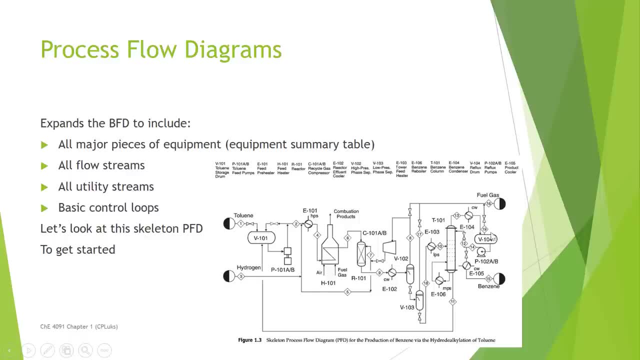 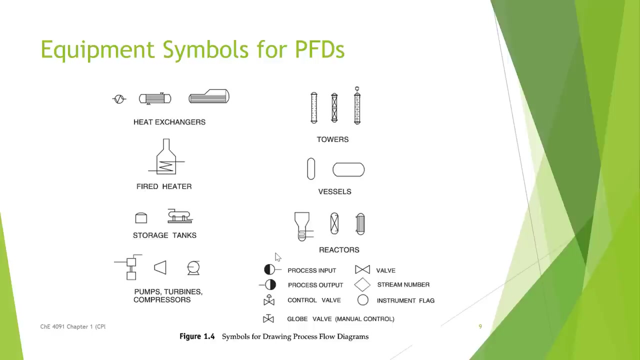 set two different ways, et cetera. Where the stream terminates is going to be a circle, with a dark right half. Where it's initiated, the storage drum, where it was fed from, is a circle with a dark left half. Some of the symbols- and there are lots of symbols that you can use- 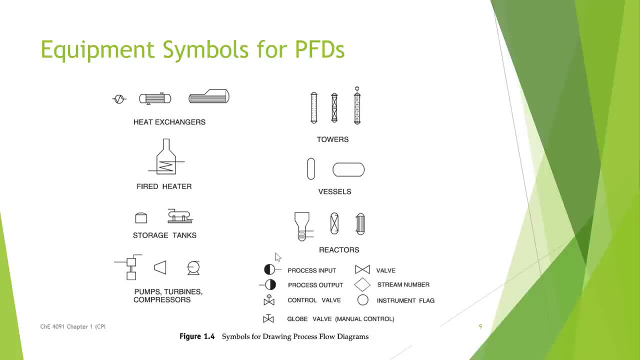 but there are lists of these in your book or various places on the web where you can look up and see what traditional symbols are. We're going to be doing a lot of our modeling using Aspen and it knows these symbols and we'll have some choices of ways that we can do these. 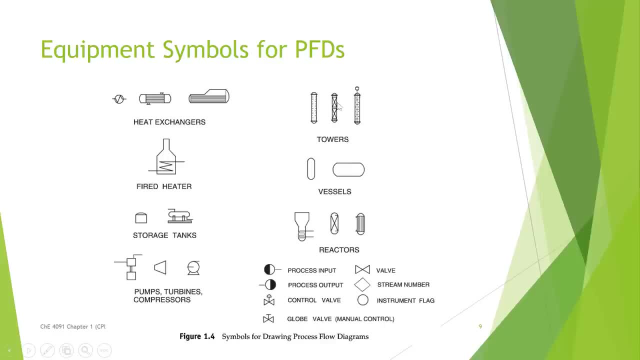 But we'll have different things, like if it's a packed tower, I'll do these little Xs, And if it's trade, I'm going to do little dashes kind of across to indicate that there are trays in there. So there are things I can do so that we actually are giving a lot of information. 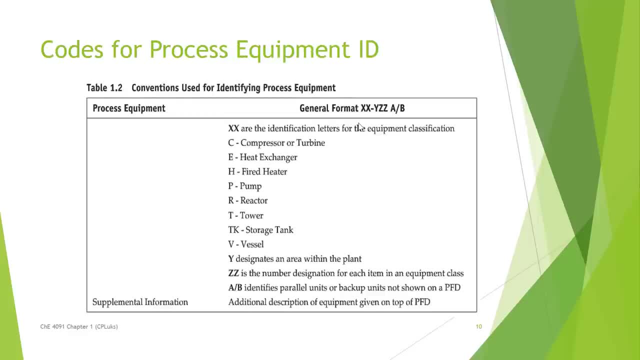 in this very simple diagram, Process equipment. we're going to be needing to name those Generally. they're going to have this format here: XX-YZZ, and then maybe an AB. The XX is identifying what type of equipment it is. So C for a compressor or turbine, E for an exchanger. 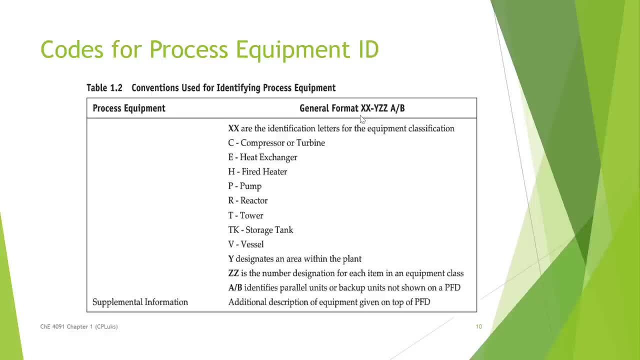 H is a fire heater, P is pump, R reactor, T for a tower, Tk, K for tank, V for vessel. A lot of times, at a particular plant you work for, they may have a different list of what letters they use. 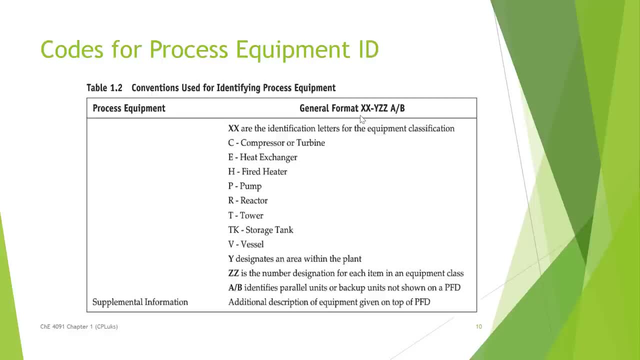 but this is what we'll use in this course. just for clarity, The Y and the ZZ are numbers that are identifying where it is. So if you have a very complex plant, the first number would indicate that it's in the olefin unit or it's in the cracker. 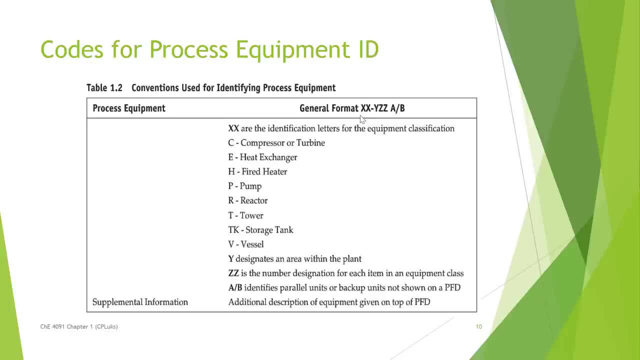 So it's telling you sort of the region, where it is, and then the ZZ is going to be further defining that AB indicates that you have, say, an installed spare, Frequently on pumps we're going to have an installed spare and so when you look at those it's going to say like P-102AB. 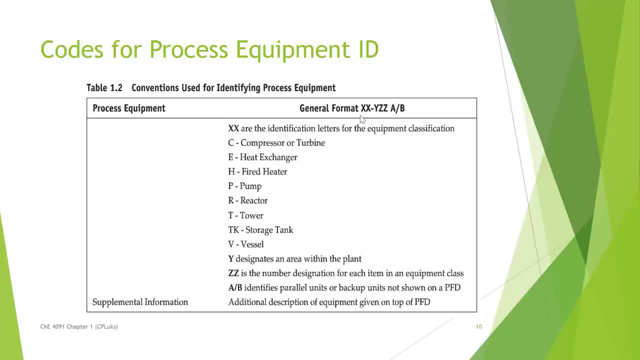 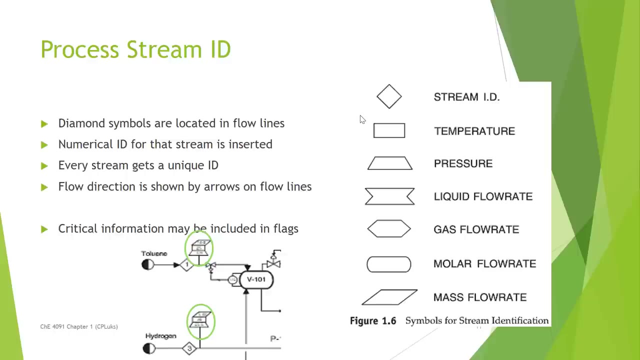 And that means that you have two of them there. only one is being used at a time, but the other one is there, So that you can never shut down because of a pump problem. You also, on critical streams, may use process stream identifiers that tell you specific information. 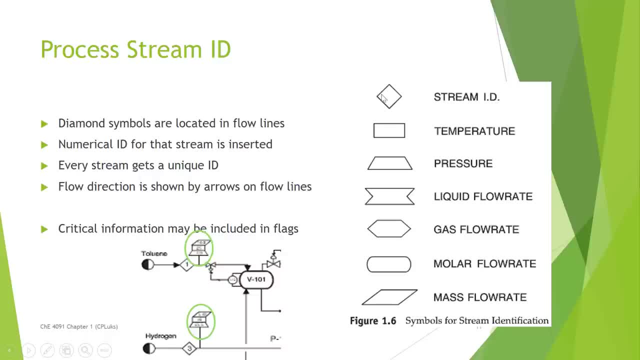 Now, normally we're just going to put a stream identifier on it, and this is what the authors of our book recommend. We'll go with just the little number blocks that Aspen does. You don't need to change those, But if you need to include flags with critical information, 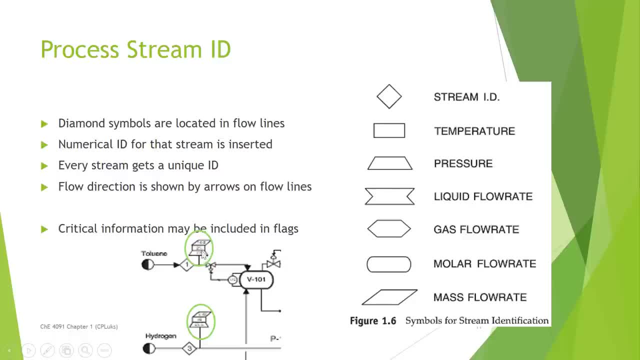 so that you don't have to say you know exactly what all the numbers inside there really mean. the shape is an indicator of what it is. So temperature: you put a number in there and then people hopefully know what the default units are for your plant. 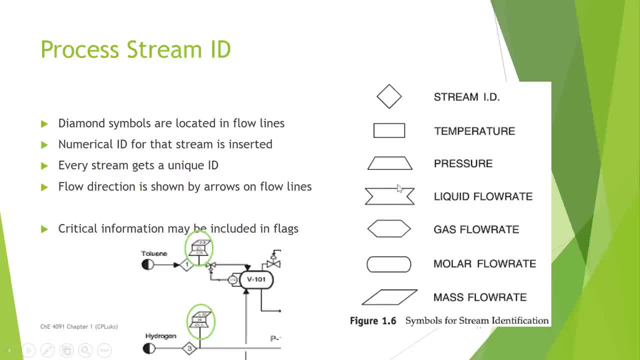 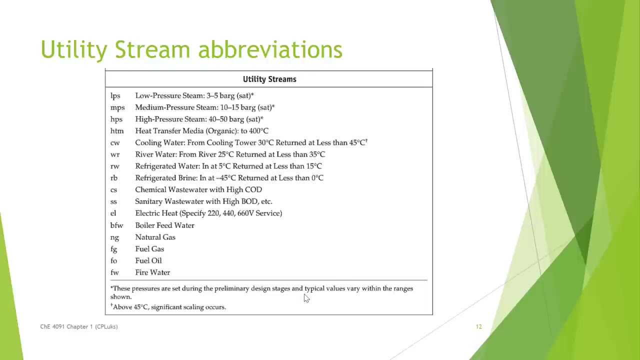 And so it saves you a lot of time and writing. if you use these standard. they look like what Dr Seuss hats: The cat in the hat, Something like that. Utility streams- we're going to have shorthand for when we talk about whether our steam is at high pressure. 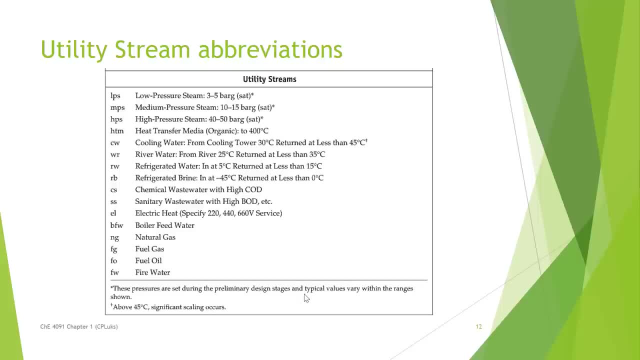 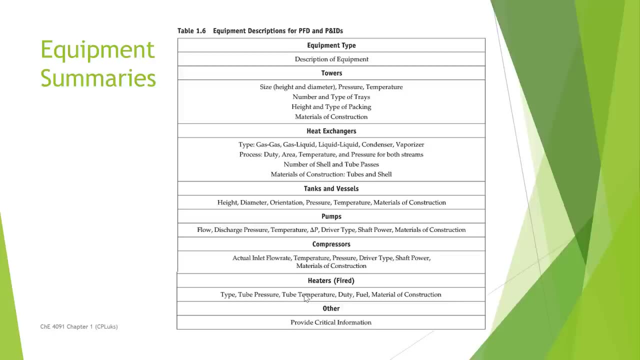 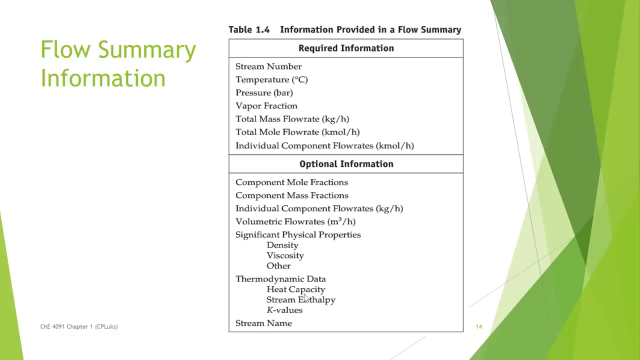 low pressure, etc. What fuels am I using on that Fired heater, etc. And then we're going to have tables attached and the tables are going to be things that are like equipment summaries or information about a plant. We're going to need a flow stream. 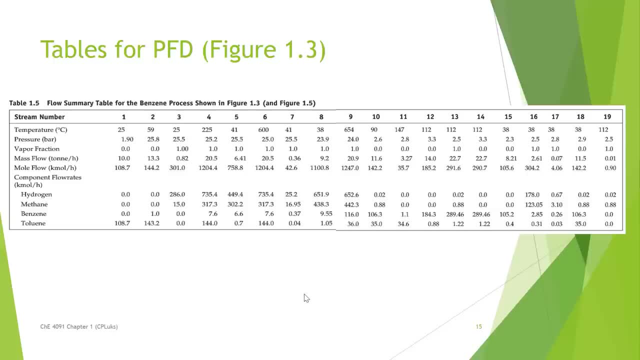 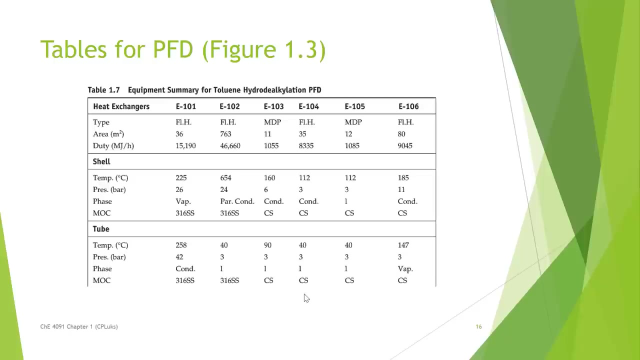 And then we'll need a table that summarizes the data, the composition and the basic thermal properties of each of our flow streams throughout the process And something about our equipment. We'll want this summarized so that I can look one place and find all of my heat exchangers, etc. 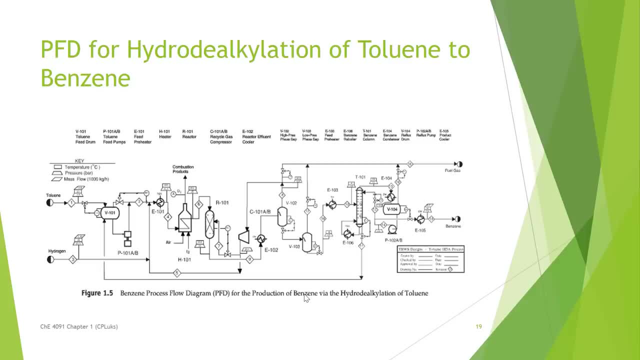 More of these. So this is a process flow diagram for the hydrodealkylation of toluene, And you'll see here that it looks a little different than the block flow diagram. A couple of places have these little indicators of key properties. 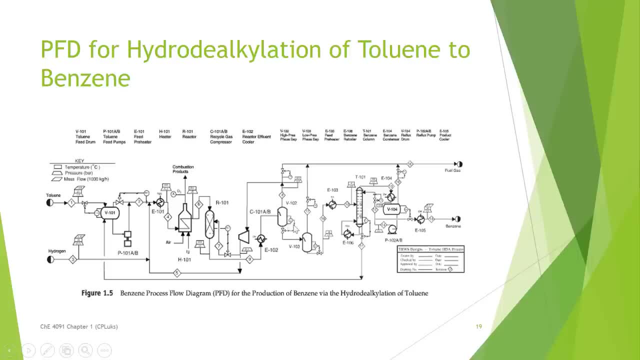 But for the most part it's just showing us specifics of equipment. It's showing me the most important of my control systems, But not all of them. Equipment is identified up here. I've got some of the basics here, But then there are also all the tables that are attached to it also. 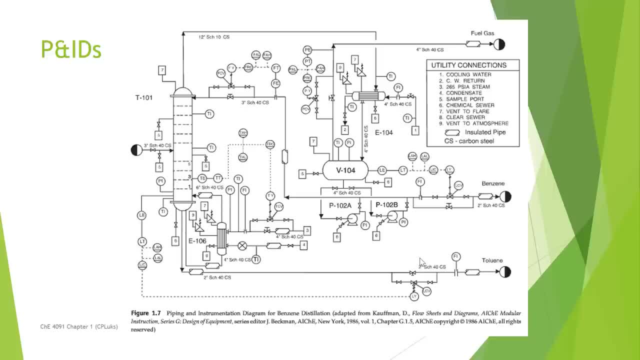 Now, a PNID has a lot of detail. So here before I just had one little loop where it was saying it was measuring here the temperature and coming down, and then that was controlling the flow. That's all it showed. This is the reality. 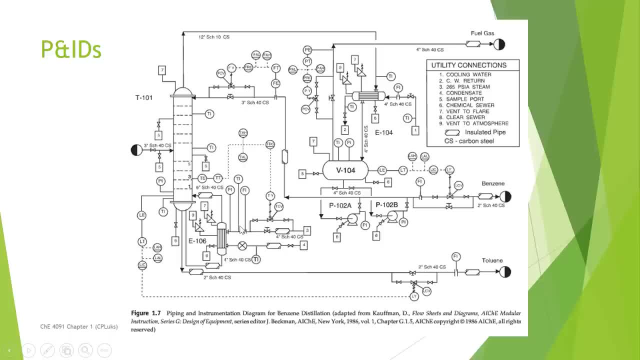 So now we've included our safety equipment here. We've included all of the lines. I've got my bypasses. This is the detail that you need so that you truly can do that final design, Purchase equipment, Make your final plans for building an actual plant. 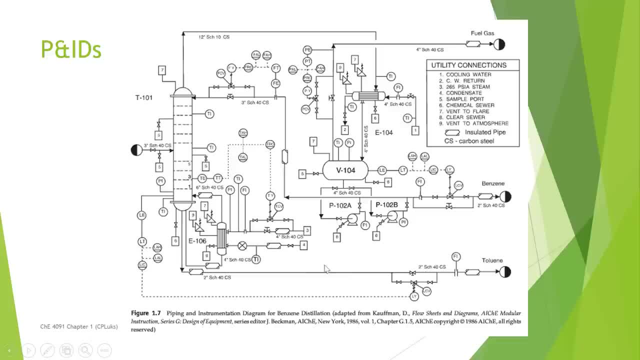 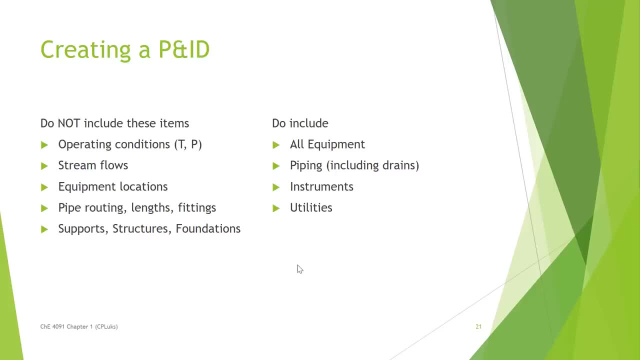 They've indicated things like pipe sizes. So all of that is critical to the final PNID. Now, when you're doing the PNID, you actually are taking some information off. So you're not going to include operating conditions or stream flow rates, You're not going to say where the equipment goes. 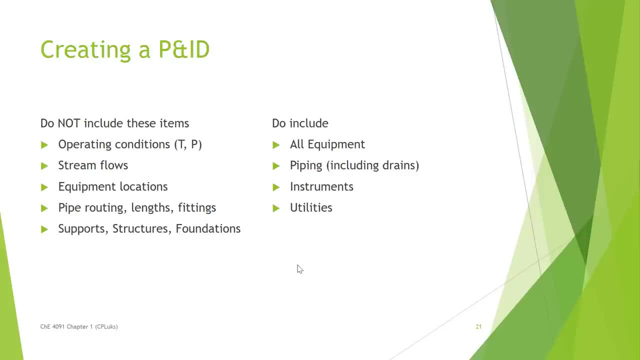 or like the pipe is going to go over the pipe rack, Not doing that stuff, But you are going to say pipe size. Okay, You're going to say what equipment it is, What instruments you're using. Where am I measuring temperatures, pressures, etc. 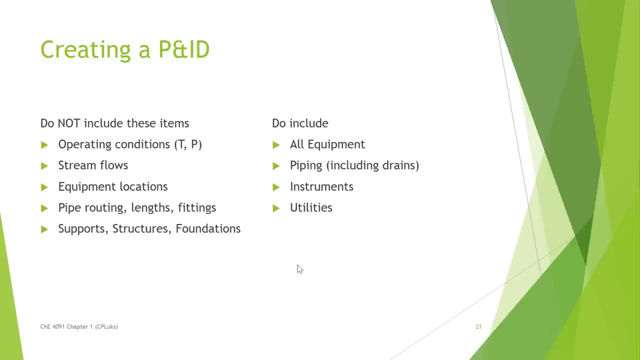 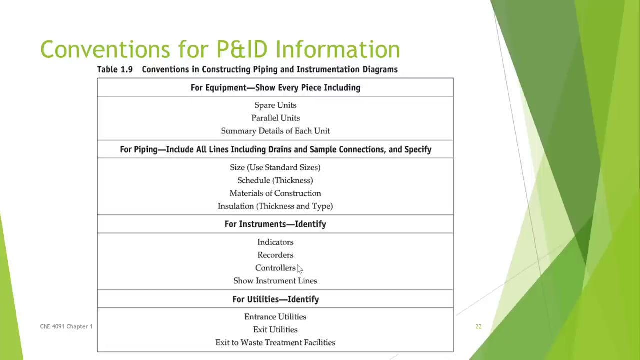 What utilities do I need Now? we'll come back to this later in the course, But just so you know where we're headed, This is really our ultimate goal for our designs. There's a lot of conventions for the information on this And again, we'll come back to this later in the course. 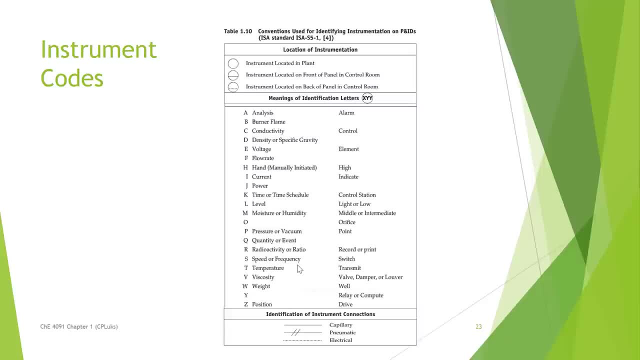 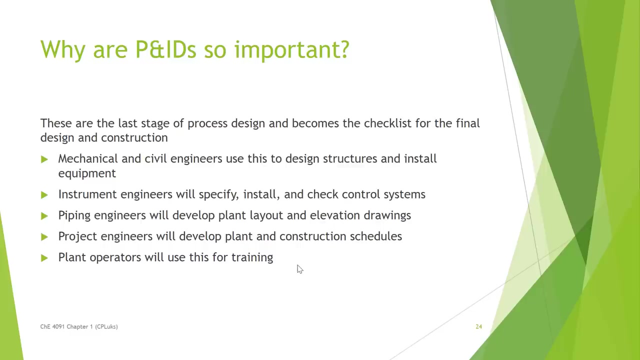 And codes for instrumentation, So alarms, transmitters, a controller, etc. And you've run into these in your controls course. Now, PNIDs are so important because this is the final stage of the design And becomes the checklist for the team that's going to do the construction. 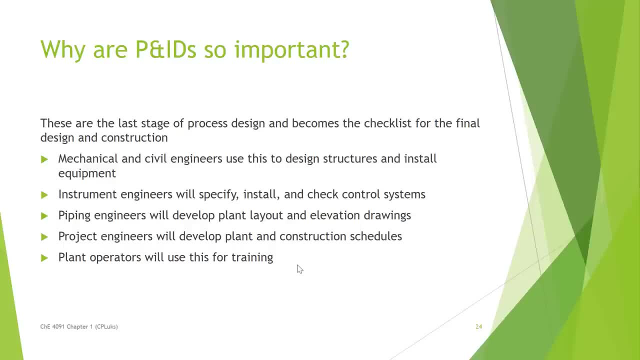 So they use this in order to get the design structures. They say: you need this and you need all these things attached to it. So therefore, when I build the structure to support that distillation tower, I need to have access at these locations. Okay, 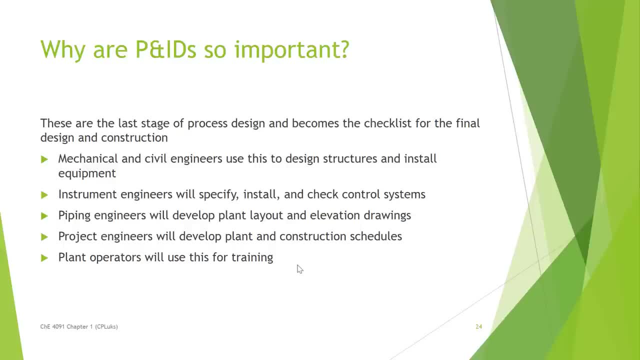 You're going to then hand this off to the instrumentation engineer, who's going to check and make sure that the control system really is valid and going to work, But also specify exactly what sizes and details you're going to need for all of that control equipment. 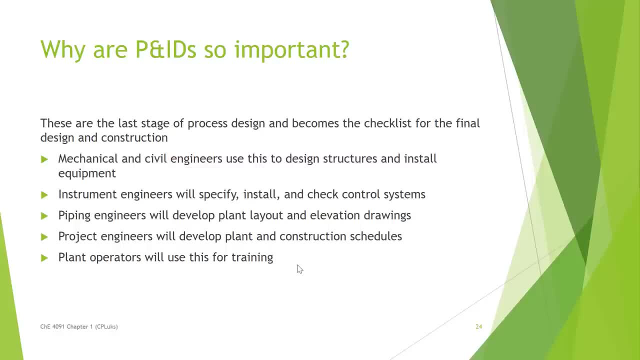 You're going to send it on to the piping people, the project people to do construction schedules- All of these are going to use this. And, finally, you're going to have a working plant and you're going to hand it to the plant operators. 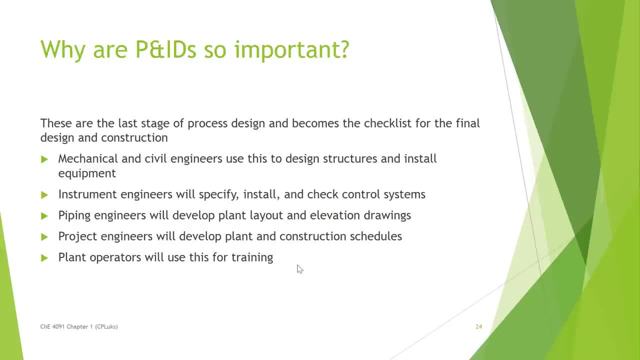 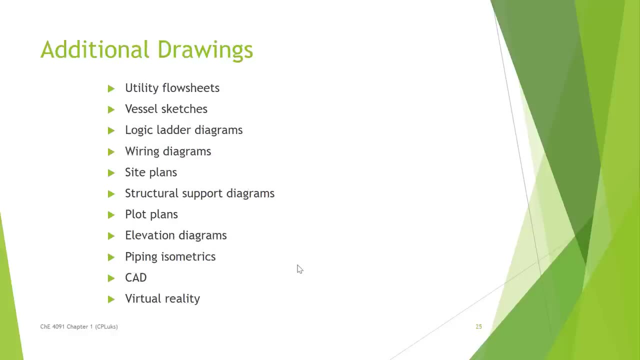 And they're going to use this PNID so that they learn how to operate the plant safely. But there are a lot of other drawings that we use, So we've got utility flow sheets, vessel sketches, logic ladders for those control systems. 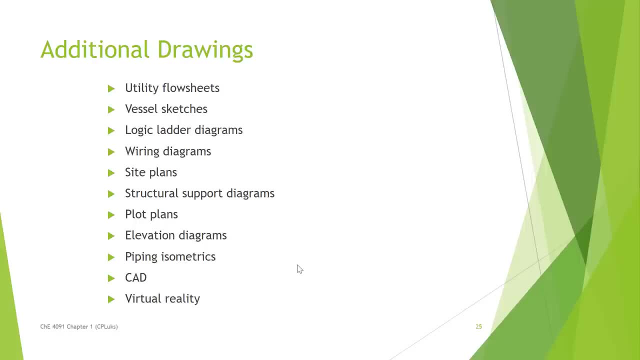 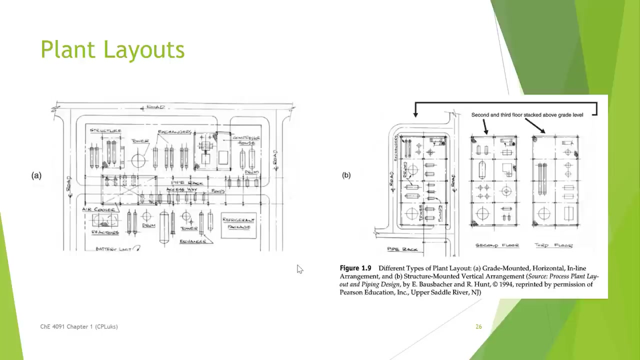 wiring diagrams, site plans, plot plans- So many. We're just going to look very quickly at some of those And, as you need them, you'll kind of learn more about these. But a plant layout is going to actually be very important for us. 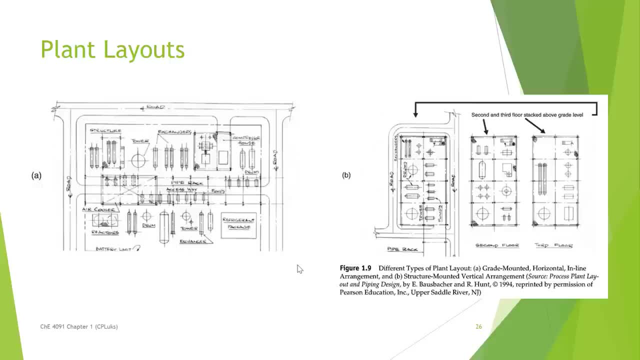 Because a plant layout shows that I can fit the equipment in the space provided. Now I may have this so that I have it all on one level, Or I may have it so that I have, say here, three levels of equipment And I want to make sure that I'm lining things up appropriately above each other. 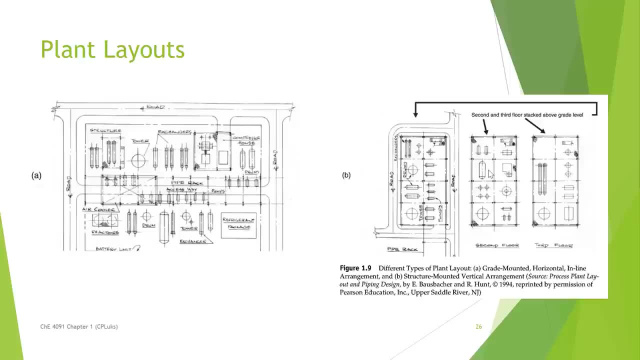 on the different levels, Because if you have to go up a catwalk and you get up there and it doesn't line up to where your access point is, Maybe you're trying to look inside a tower And the access point is not where the catwalk took you. 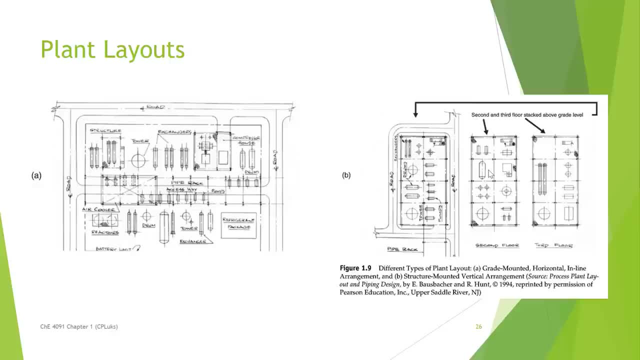 Then that's a bad design, So we need to have that. But heat exchangers, Shell and tube is a very common design. I want to make sure that I'm leaving enough space so that I can pull out the tubes if I need to do any repair work. 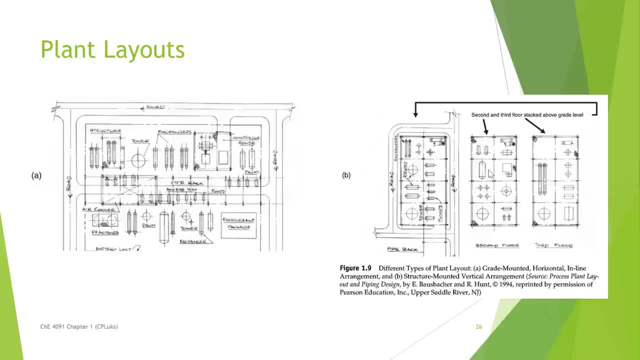 So these are the kinds of things and reasons we do a plant layout. I also want to make sure that things are far enough apart so I can work around them Or so that I can operate them safely. There are some recommended spacing between process equipment. 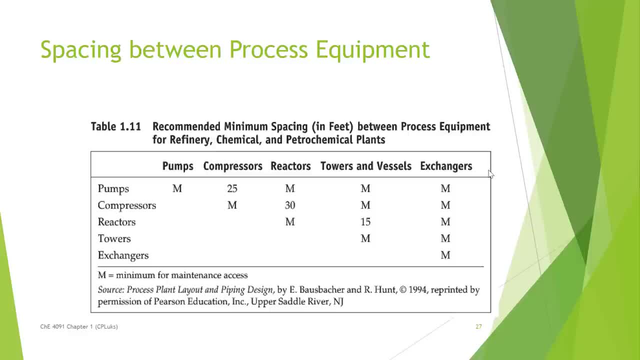 M means just the minimum, so that you can get bodies around them, But these others are number of feet. So pumps and compressors should be 25 feet apart. Reactors and compressors should be 30 feet apart. So these are some things that we need to keep in mind. 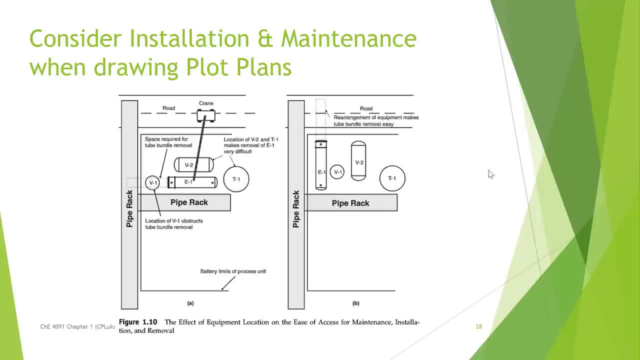 And then again reminder that you need to have space, This heat exchanger here, if you wanted to pull the tubes out. it's got a vessel there, So every time you had to pull those tubes out you would have to remove this vessel. 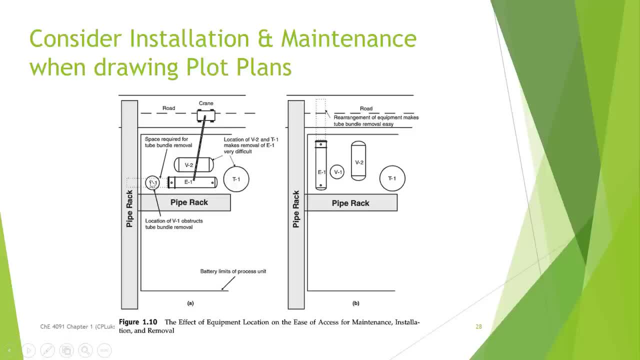 then pull the tubes out, do your work, put them back in and return this vessel, Or you could just reorient this so that now, then, you have the roadway. All you have to do is block the road for a few minutes until you pull this out.